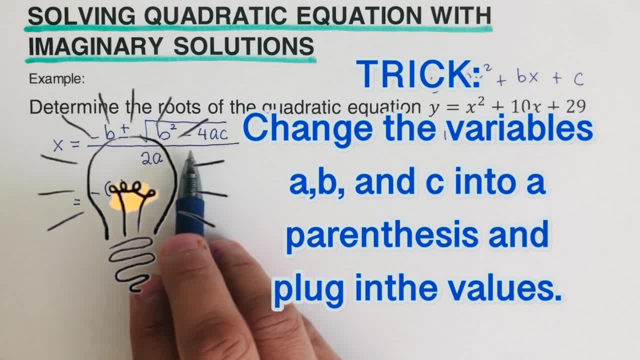 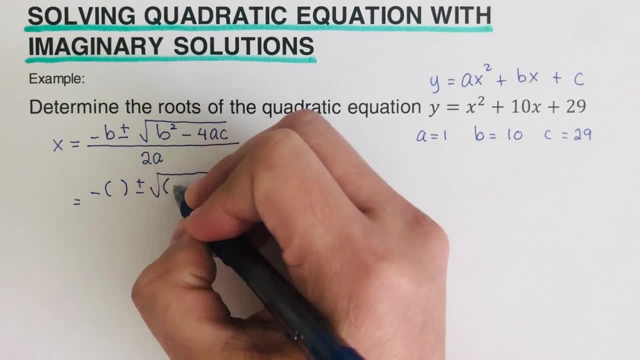 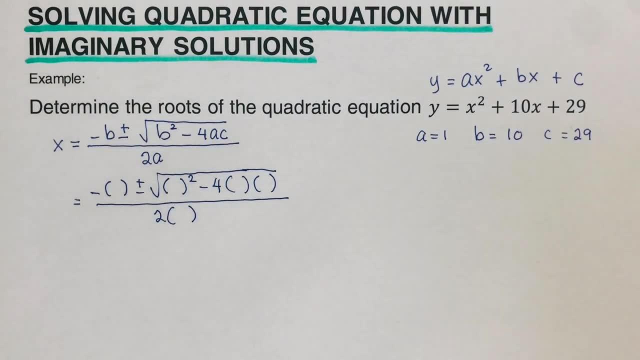 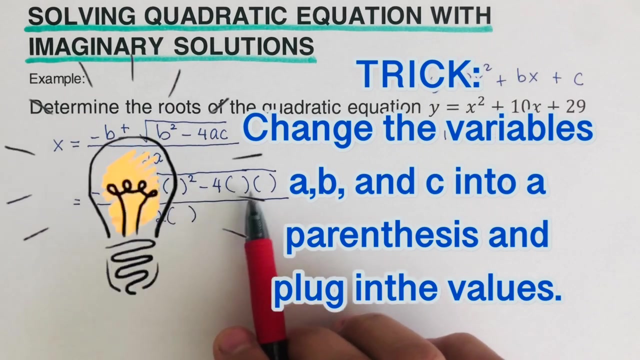 I will change all the letters into a parenthesis before I plug these values in. Okay, so that's the trick, so that you don't mess up with the math. So the trick here is that you change all of the letters into a parenthesis first, before you plug. 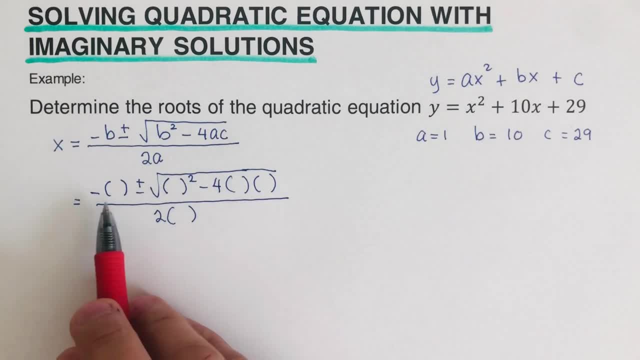 in these values. So then, after we're done putting the parenthesis, we are going to plug the values in. our b is 10, so I'm going to write 10 right here. Our b is another 10, so I'll write the 10 there. 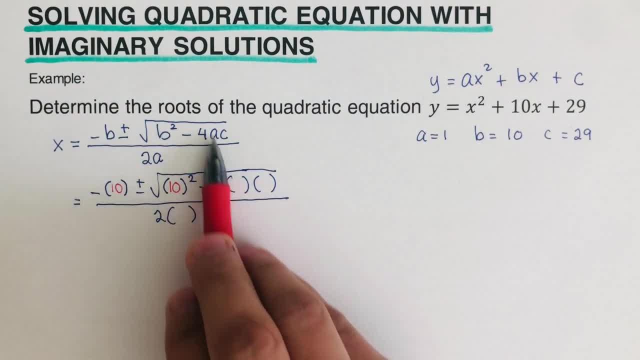 and then our a, so this parenthesis matches up with a and that is a 1. and then our c is 29, so I plug that in here. and then our a is 29, so I plug that in here. and then our c is 29, so I plug that in here. 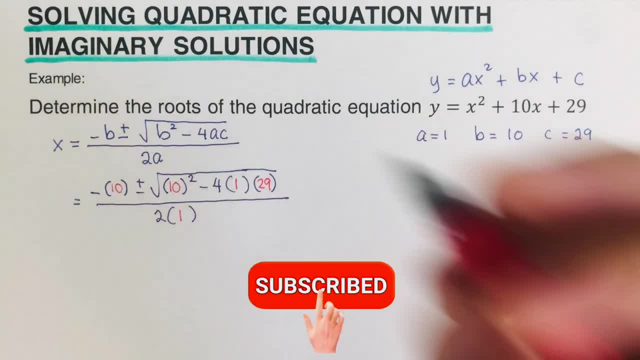 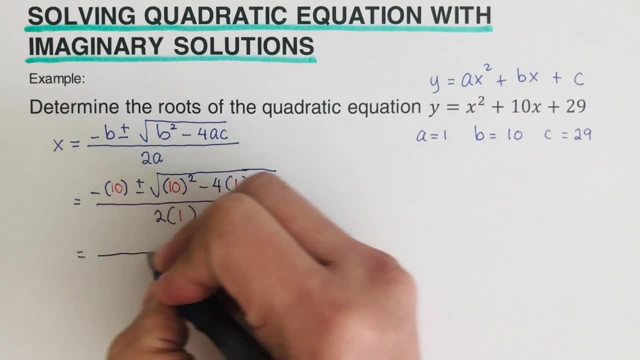 Our a was 1, so I put in the 1 here, and so we are going to simplify this. So this would come out: that's the negative of 10. would come out a negative 10.. So that's a negative 10 plus minus. 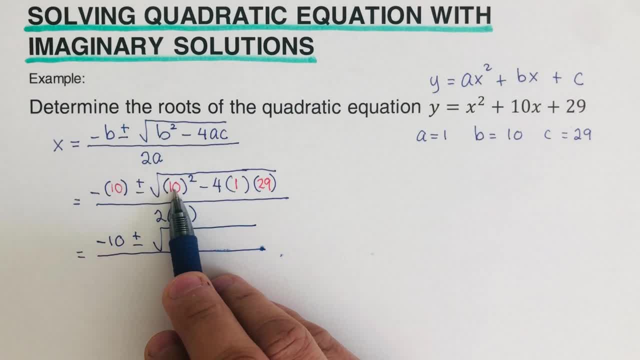 square root of that's going to be 10. squared would be 100, so I'll put in 100 right here. minus 4 times 1 is 4 and then times 29 is 116 and that is divided by 2.. because 2 times 1 is 2.. Now notice why I had to change this into a parenthesis, because others 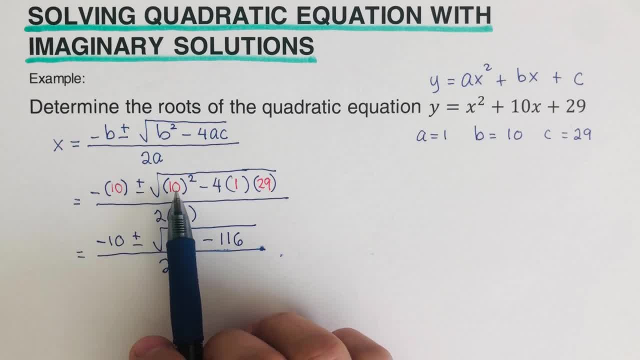 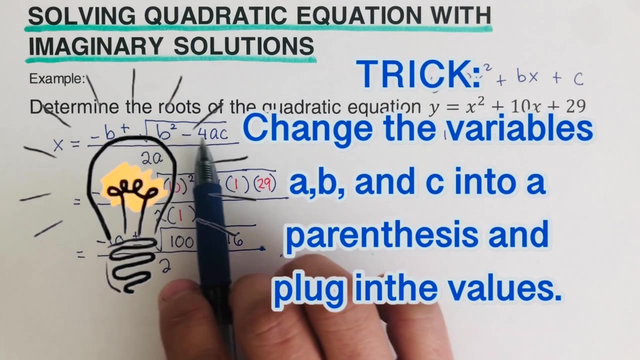 miss this part when they, when they don't use this trick that I give you to change this into a parenthesis before you plug in values, they're going to have trouble doing, especially if the values have negatives on them. So again, the trick is change all the letters into a parenthesis. 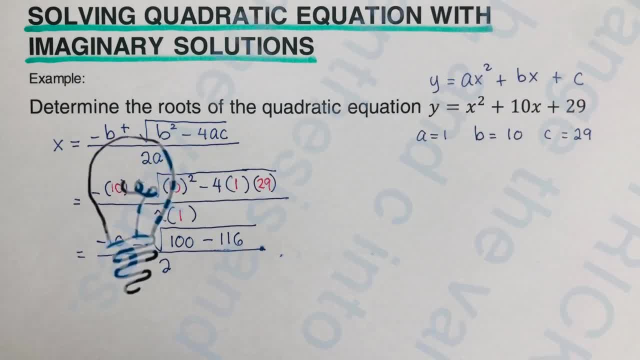 before you plug in a, b and c into it. So then from here we can go ahead and simplify this. So we start with the ones inside the radical right here. So this can be written as negative 10 plus minus square root of that's going to be a negative 16 and that is over. 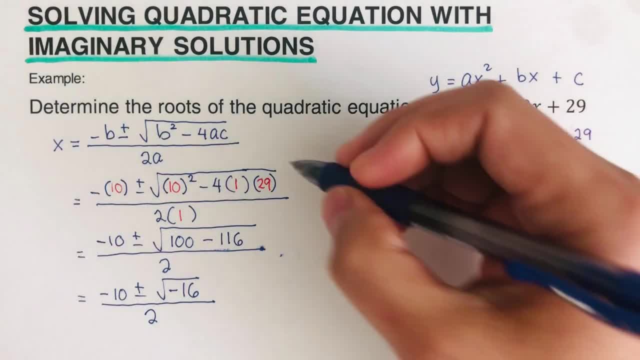 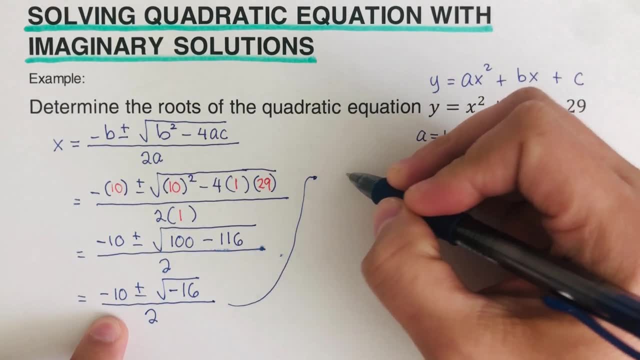 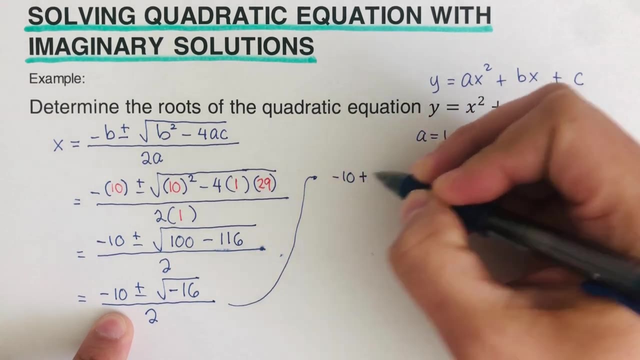 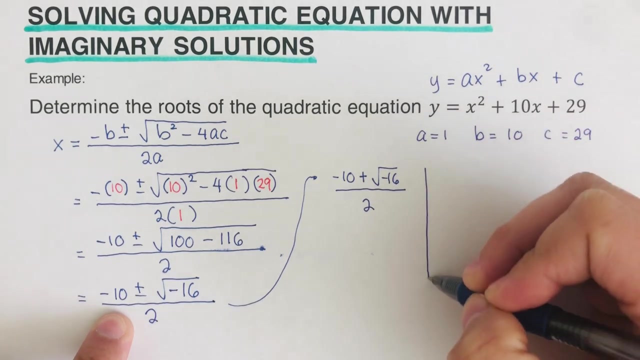 2. So then we can go ahead and divide this into. I'm just going to show the work up here So we can actually divide this into two parts. So the first one is that's going to be negative 10. plus square root of negative 16 over 2, and then the other one is the minus part. So it's pretty. 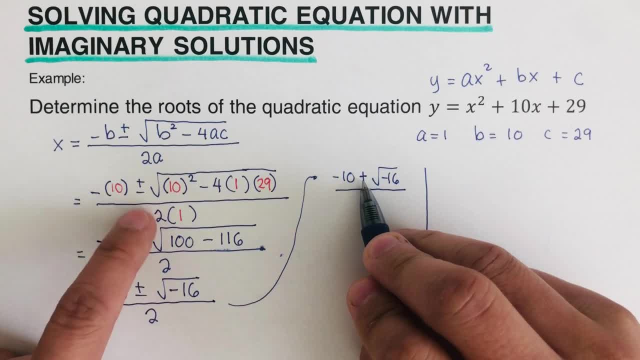 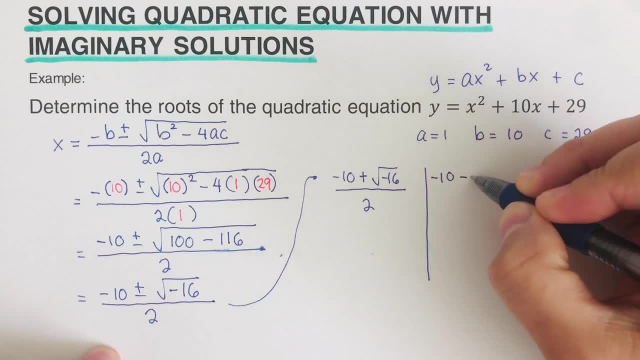 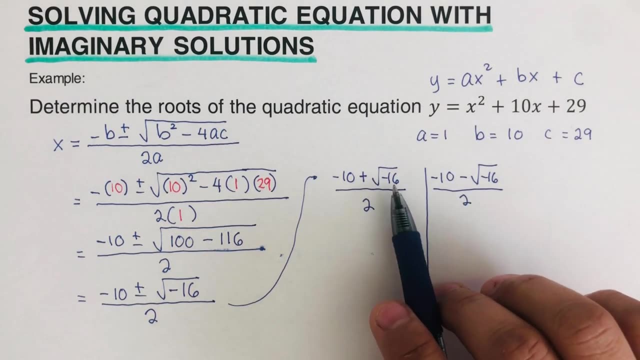 much the same thing, but this is going to be a minus. remember that's a plus and minus, So I'm breaking it down into two parts, the plus and the minus. So that is negative 10. that's minus square root of negative 16 over 2.. Please remember that square root of 16 is 4 and since there's a negative, 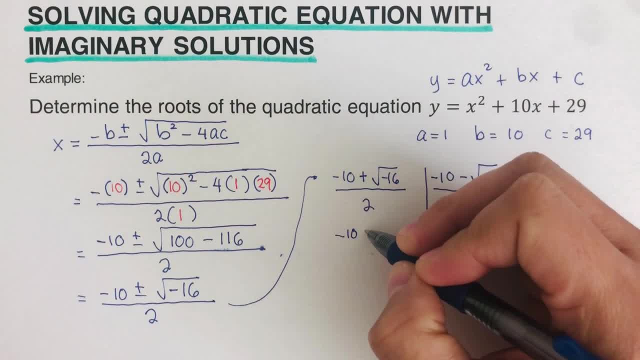 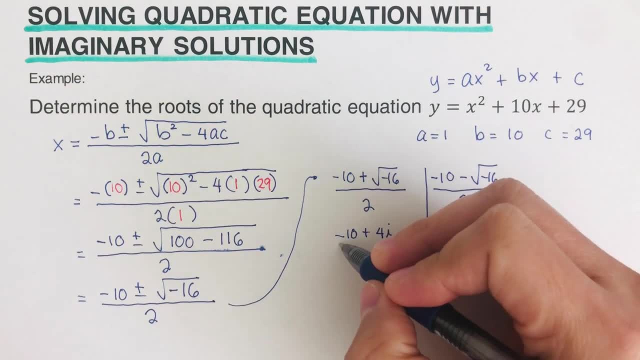 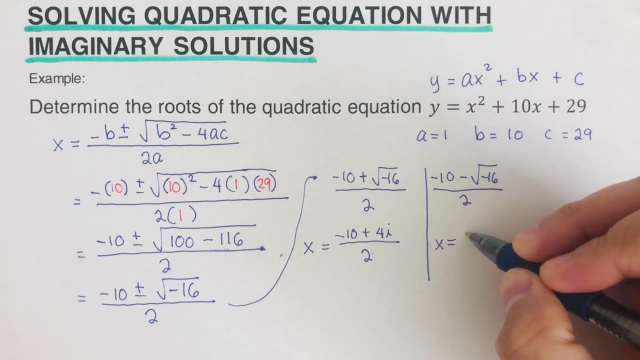 so I put an I, So this comes out negative: 10 plus 4i. So again, square root of 16 is 4, and then there's a negative, So I put an I, that's over 2.. This is equal to x. and then the other one right here would also be negative: 10 minus 4i. Again I write the 4i, because square root of 16 is 4, but there's a negative, So I put an I and that is over 2.. Now please remember that the 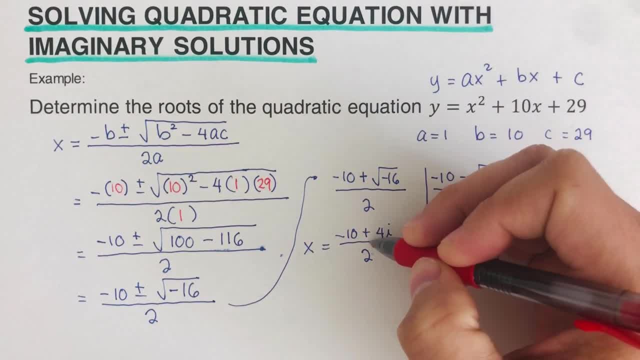 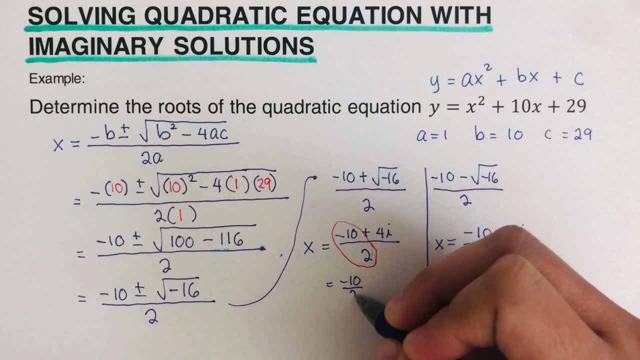 this 2 is shared by both of them, so the 2 is the denominator of negative 10. so i can go ahead and rewrite this as negative 10 over 2 plus, and then, at the same time, this 2 is the denominator of 4i. 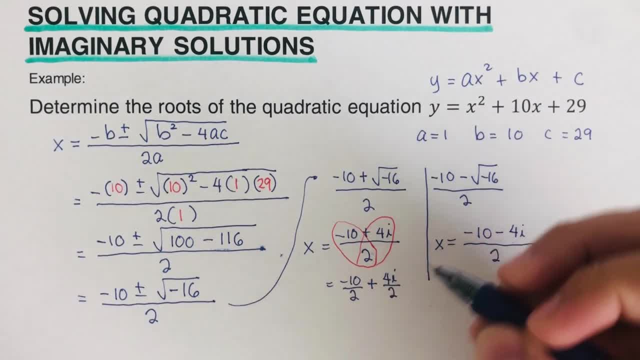 so that would be 4i over 2. so i can simplify this as negative 5 plus 2i, because you have a negative 10 divided by 2 is negative 5 and 4i divided by 2. so 4 divided by 2 is 2, and then we put the i. 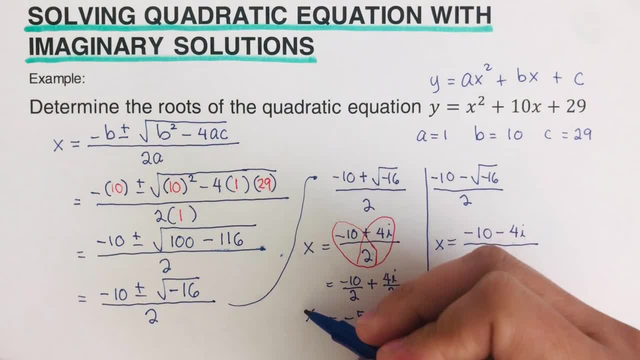 so this is our first x, so this is our first root, and then the other root would come from this. so then we go ahead and um rewrite this as um again. remember this: 2 is the denominator of negative 10, so that is negative 10 over 2 minus, and then it's also a denominator for negative 4.